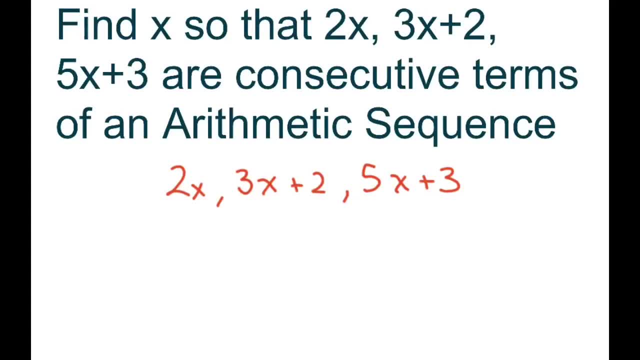 Hi everyone. we're going to find x, so that 2x, 3x plus 2, and 5x plus 3 are consecutive terms in an arithmetic sequence. So basically, this would be our first term, our second term and our third term. 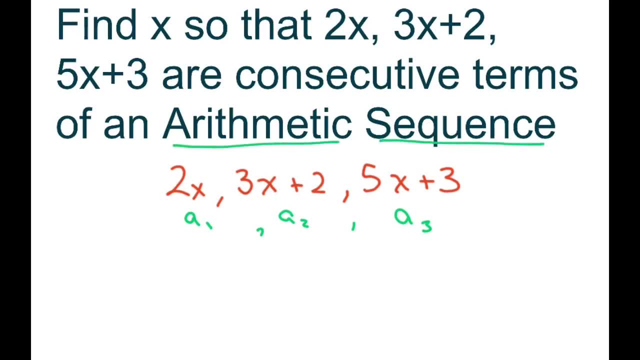 And what we know about arithmetic sequences is they have a common difference. So whatever the common difference is between those will help us solve for x. And then we're going to find the common difference and find also use a system of linear equations. So basically to find a common difference. say we have 5,, 10, 15, our common difference, you can see clearly, is just 5.. 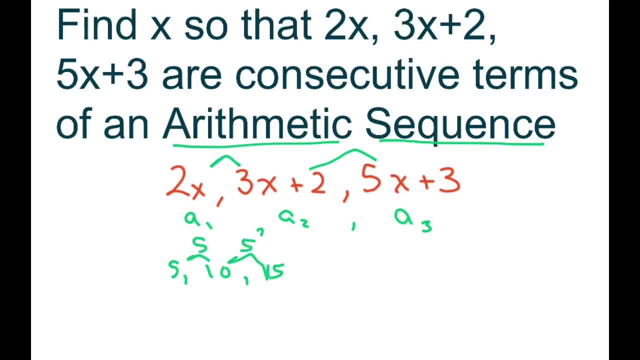 And what you do is you subtract, that's 15.. What you do is you just subtract. You subtract the term you're looking at minus the previous term. So 10 minus 5 equals 5, or you could do this one: 15 minus the next term. the previous term would be 10.. 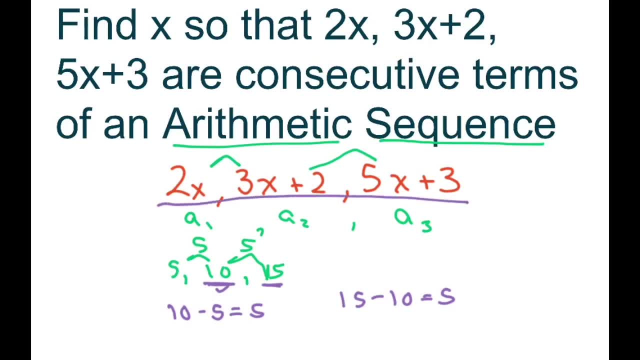 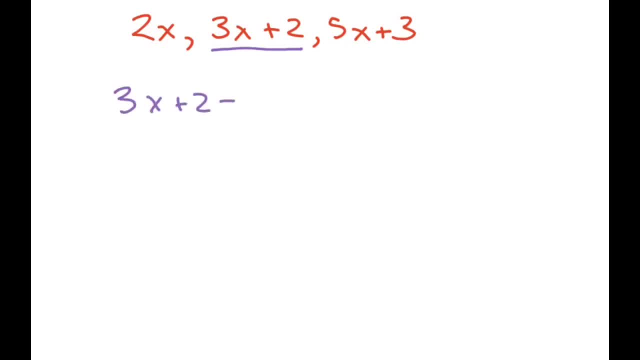 That gives you 5.. So that's what we're going to do with those. Then we're going to form a system. So I'm going to take this term minus my previous term, And that's going to be 5.. And that's going to give you x plus 2.. 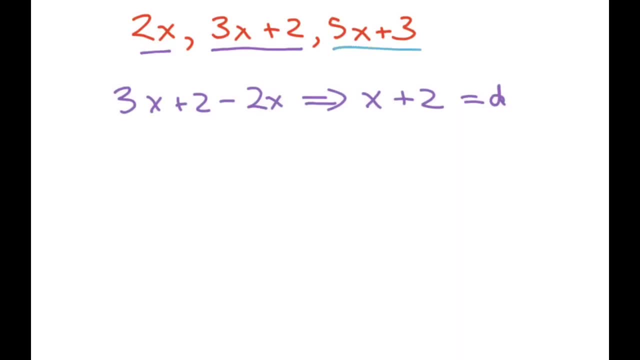 That equals your common difference. for that Now we're going to do this one. I'm going to write 5x plus 3 minus 3x plus 2.. And when you distribute this negative here, you're going to get 5x plus 3 minus 3x minus 2.. 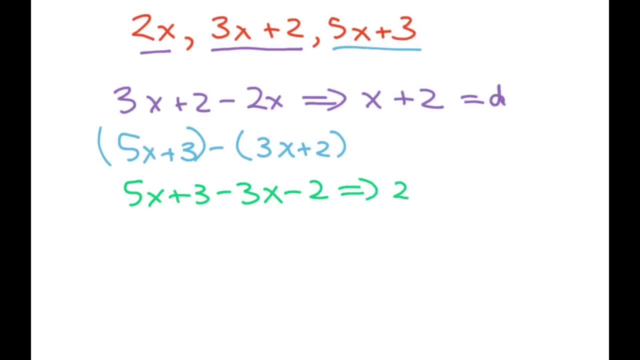 And that's going to give you a 2.. And that's going to give you a 2x plus 1.. And that is your common difference. So now we have a system of linear equations, So we have d equals d. So I'm just going to set my d's equal to each other. 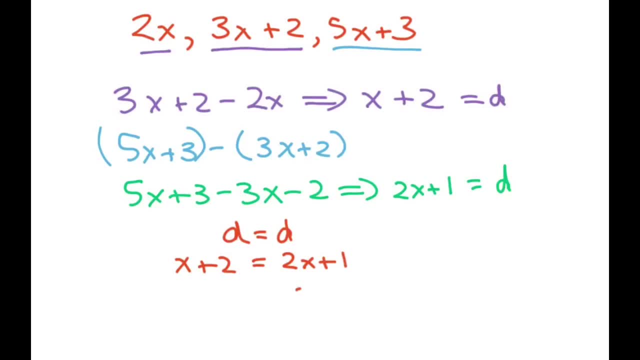 And solve for x. So that's going to give you x equals 1.. And that's your term. Now that's your x. That's what our goal was to find that. And if we want to plug 1 in, we can see: if you plug in 1 here, you're going to get 2..